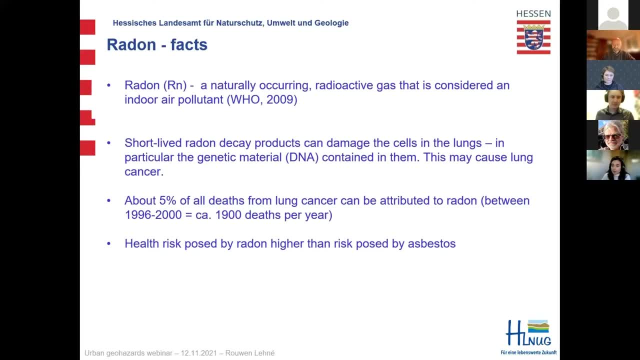 are aware of, But radon, almost no one is talking about it, At least in Germany. I know it's different than other countries- Scandinavia, That's, that's different. But as geologists we know that that radon appears in almost every: every rock, every soil And, in the end, the measurable 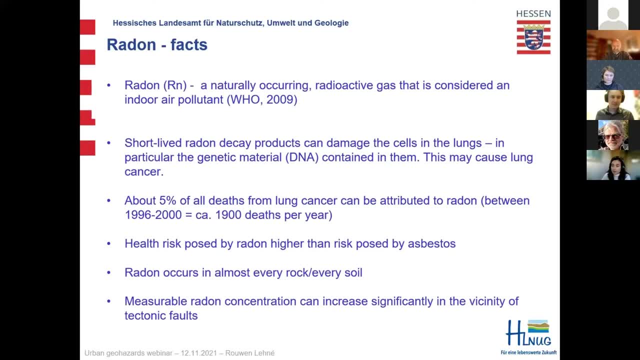 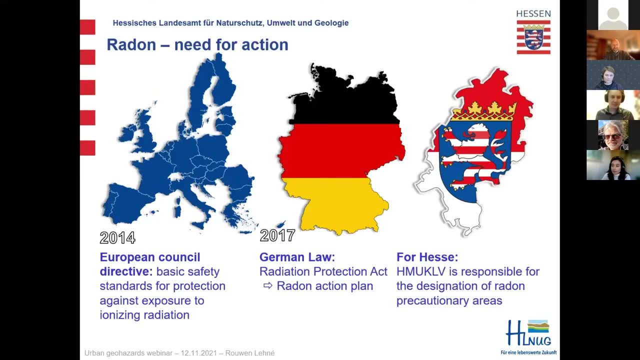 radon concentration can increase significantly in the vicinity of tectonic faults. That's something given, And that's why the European Union was looking for some action. In 2014,, the European Council directive has been established, Where it's about the basic safety standards for protection against exposure to ionizing. 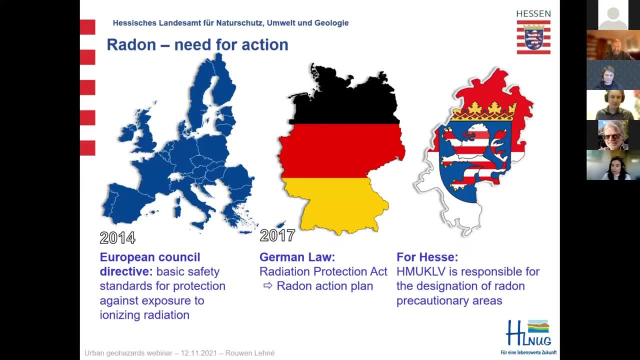 radiation In 2017, then in Germany, the according law has been established- The Radiation Protection Act- And there a radon action plan was requested by the federal states, And that's why HESA is given here, because I'm working for the geological survey of this. 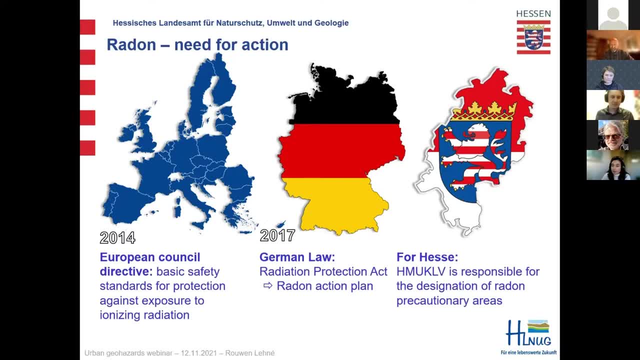 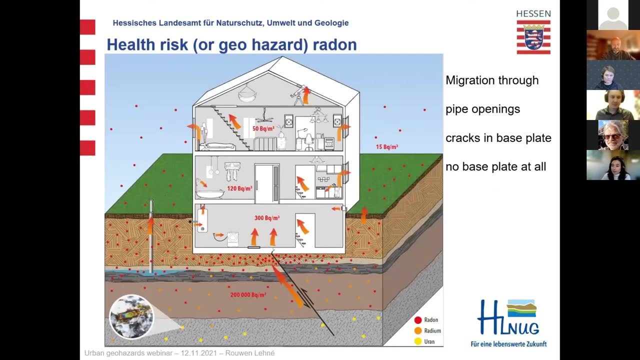 federal state. So for our federal state, we need to designate radon precautionary areas. That's what the task is. The question now is: why is this a task And what is a radon precautionary area? This is some sketch that is intending to describe the dependencies. 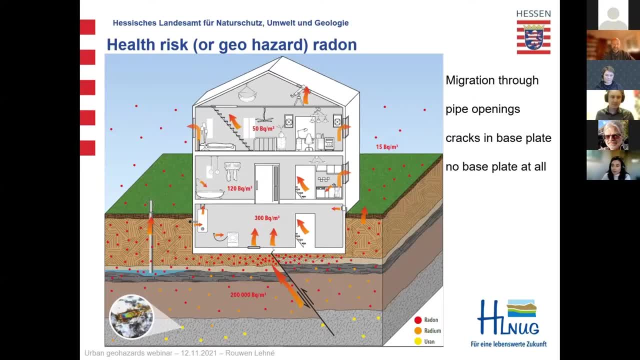 The health risk coming from radon or the geohazard related to radon. As geologists, we know about the subsurface. We know that there's a lot of of rock around and soils around- different rocks, different soils- But they all have in common that they contain. 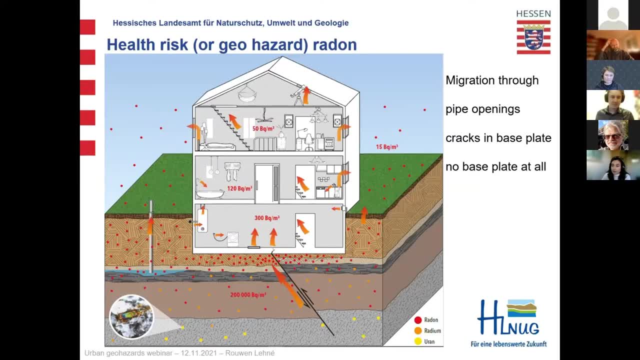 uranium. Some rocks more, some rocks less. Uranium is is the mother nuclei of the in the human body, the nucleus, the nuclear nucleus. The nuclear nucleus is the function of the radon. The radon contains uranium, So uranium contains uranium. Uranium contains uranium. 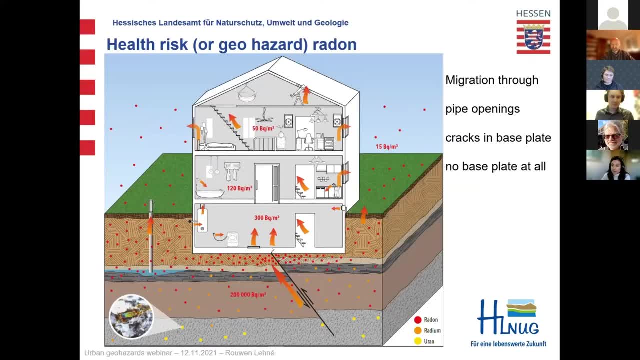 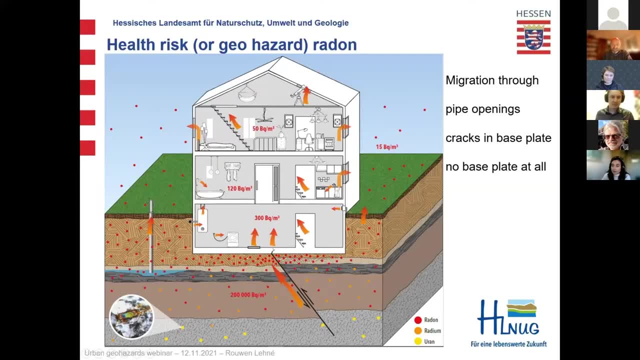 cracks in your base plate, or if you have maybe no base plate at all, that's, that's quite, quite common, quite happens quite often. or if some pipe openings are not, are not tight enough, and then radon can get into the building and the concentration can increase up to 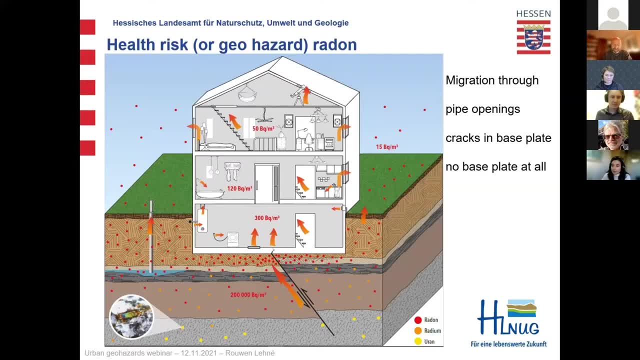 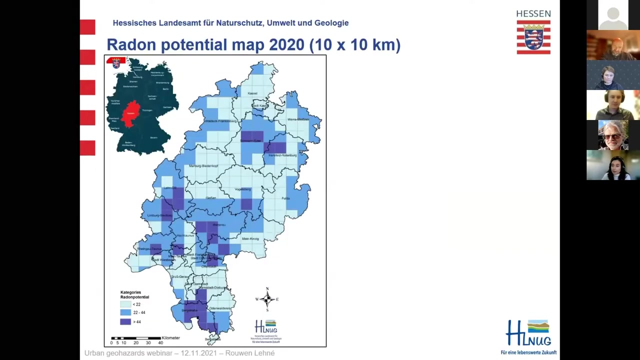 yes, significant amounts. i will show you some examples later on, but that's that's described here. so we do have an interaction between the building, the construction and the surroundings: soil, the subset of construction, growing the rocks, and that's what the problem is about. so the radon precautionary areas, they have been, they have been assessed or developed. 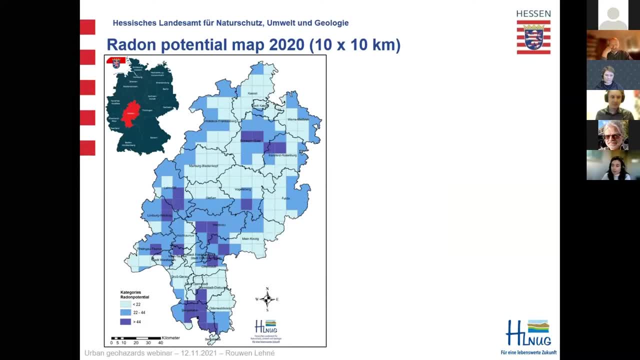 using a so-called radon potential map. this is something which has been modeled by the federal office for radiation protection in germany, and they're used for this map- soil air measurements, permeabilities and indoor measurements- and what you can see on the map is three colors, and every color is representing a category. 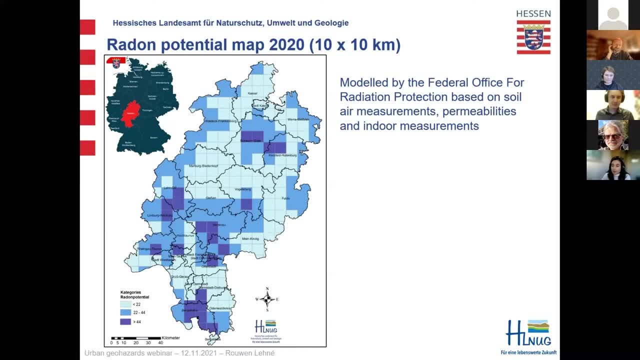 the the bright bluish color is showing a potential of less than 22, and then we have for the middle one, which is 22 to 44, and the dark bluish colors. they represent potentials higher than 44. i don't know, but i think that something comparable should have been done. 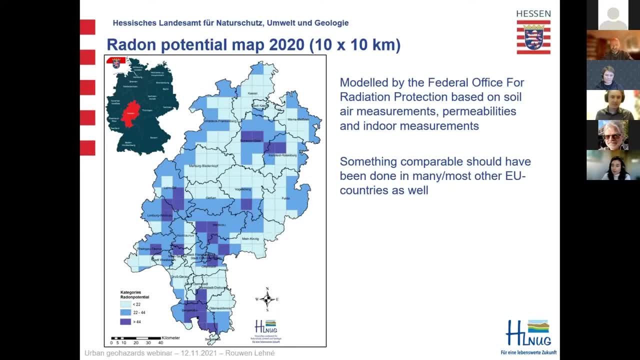 should be available for for most of the other european countries. so what does it mean in the end? you can see the federal state, you can see the counties and you can see the distribution of these tiles: 10 by 10 kilometers each tile, and only those counties have been made, would have been made a radon precautionary area. 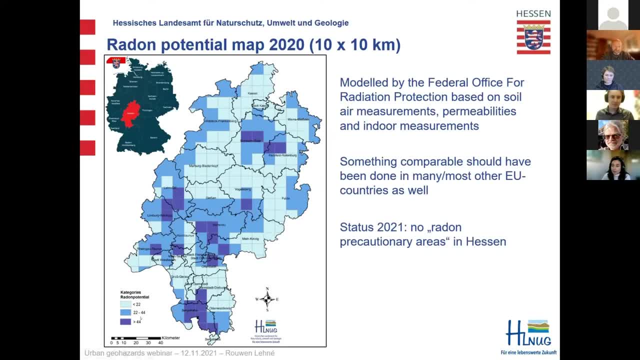 where the percentage of those tiles with a potential higher than 44 are exceeding is exceeding the 75 percent of the total area of such a county, and this is not given in any of the counties. so even if there are some tiles where we do have a high radon potential, where we do have the risk, 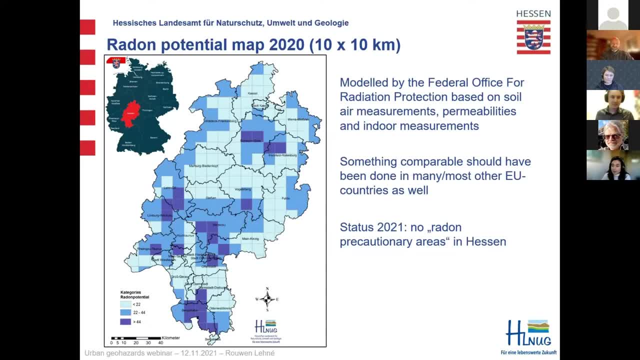 that that the average radon concentration in the room air is exceeding 300 becquerel per cubic meter per year in the average, even if we have such such areas, given the overall area which is the county, has not been made a precautionary area. so the reason why we're saying yes, but in the end this is just statistics, they it's a good model. 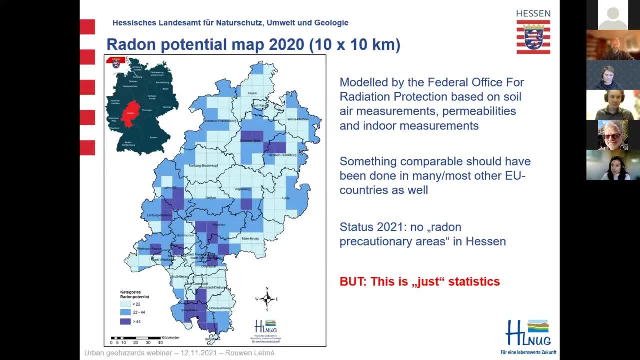 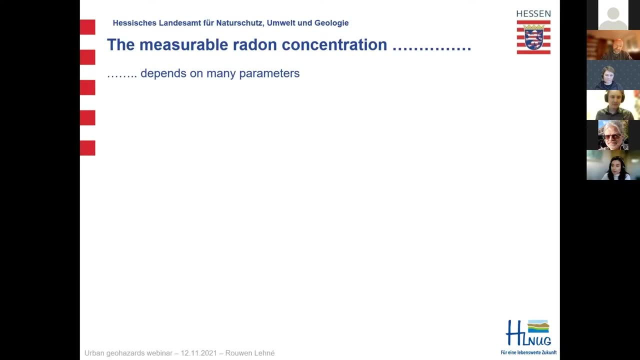 it's useful, it's help. it's helping a lot to to make people more sensitive and to focus our works and given areas where we need to get more understanding. but it's statistics. so if we're talking about the statistics we can, we can uh switch to maybe the reality and the reality. 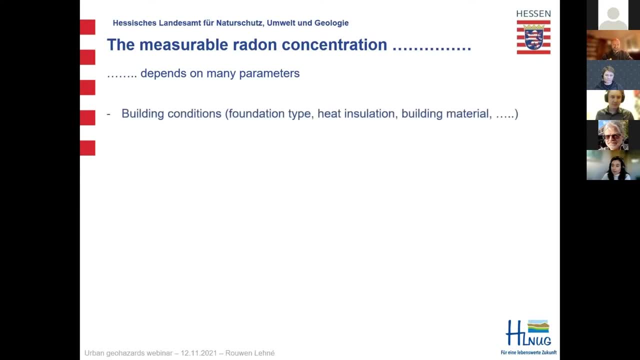 is much more difficult, in that the measurable radon concentration depends on many parameters, and something we already have seen is the building conditions, the foundation type. is there heat insulation yes or no? what about the building material? then, of course, the metrological conditions are influencing what we can measure: the temperature, 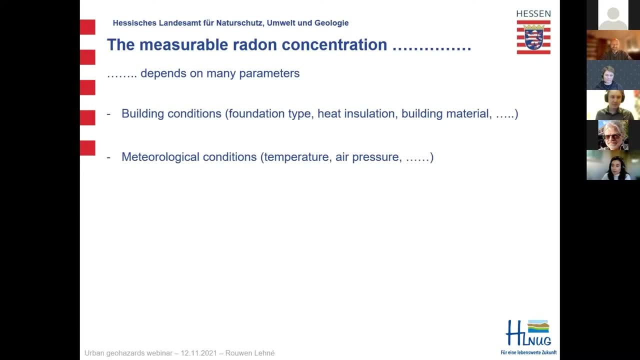 has an has an impact, like the air pressure and, of course, the subsoil. so the measurement environment is impacting a lot. what we can measure, it's the geochemical composition of rocks and soils, it's the permeability, it's the tectonic inventory and soil physics, while the building conditions are easy to assess. 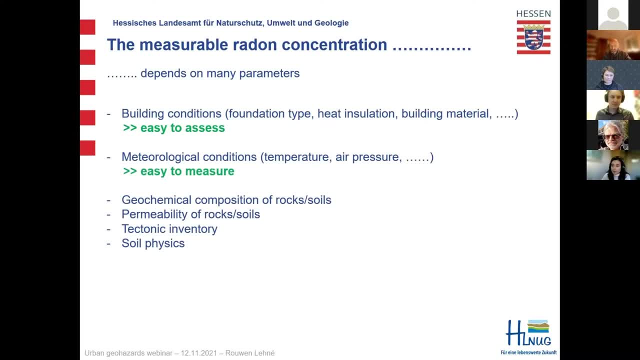 and the hydrological conditions are easy to measure. we do have the subsoil, the, the underground, as the most difficult part in this, in this context, and at the same time it's the most important one, i would say, from a geological point of view. of course, others say 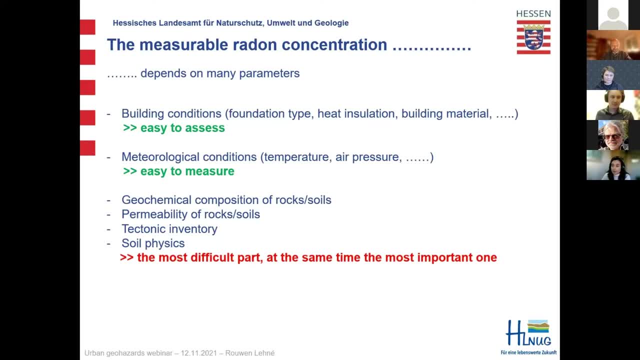 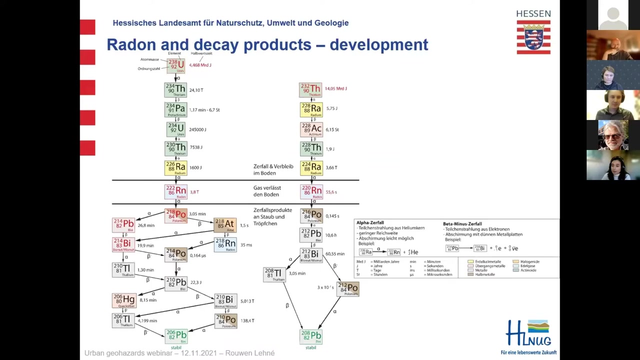 who cares about the geology and the rocks and all the uranium and radon that is that is given there? as long as we have all the capabilities to build proper buildings, then we don't- we don't have need to care about this at all. but the reality is showing us something different. the development of 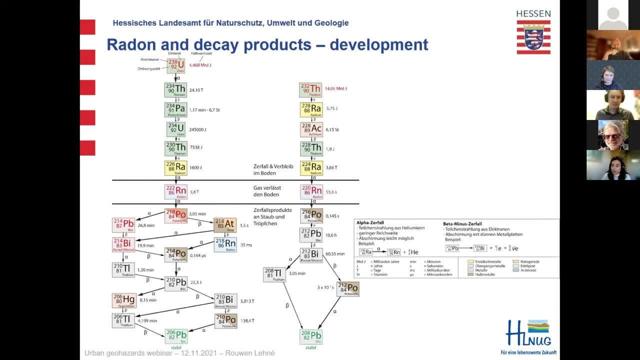 radon is given here. that's, uh, the decay chain, and down there, you see, it's the radon 222 with a half life of 3.8 days, and it's not the radon itself, it's, it's the decay products which are causing. 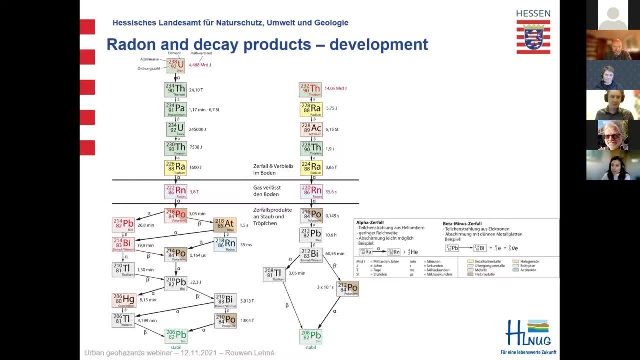 the problems because their um, their decay happens after three minutes, which is polonium, after 26.8 minutes, which is um, uh, lit. and then we have bismuth with the 19.9 minutes. and if you're inhalating those heavy metals, and if they are, if the decay takes place in your lung, then we 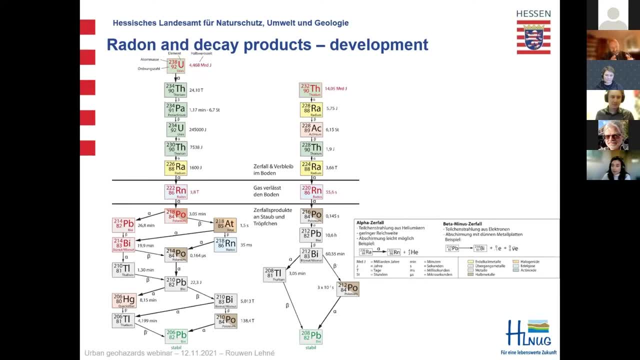 get the damages we are talking about. so it's it's not the radon itself, it's more the decay products which are which are causing the problems. but radon is, uh is the element we need to measure, is, or is maybe the only one that is? 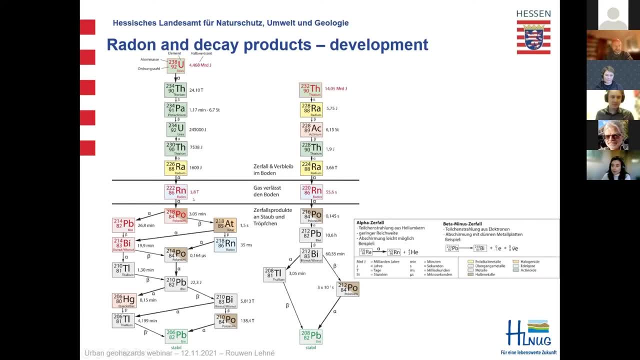 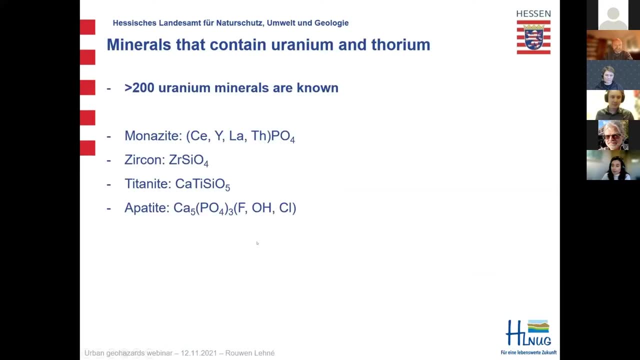 useful to be measured because of uh, its relatively long life of 3.8 days. the others are difficult to measure. that's why we focus on radar. so we we know about more than 200 uranium minerals, um and and most of them are not not relevant, but some are like monocytes corn. 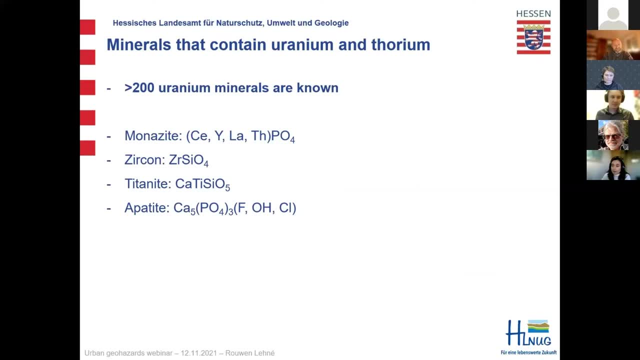 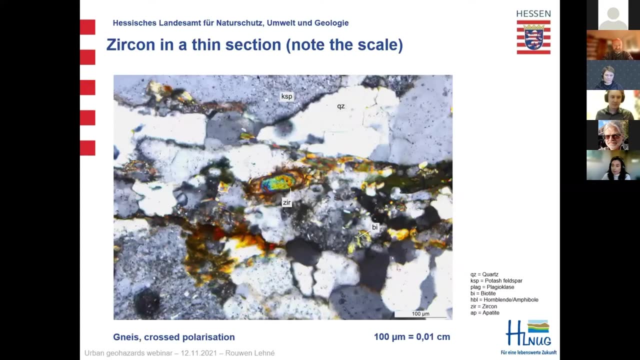 titanite and appetite. there, some uranium is substituting other components of the minerals and in a thin section it probably looks like this: we have some zircon there and some bismuth there, and it's it's almost not to see. that's why i was stating something like the scale: it's just 0.01 centimeter, which is, yeah, very tiny. it's. 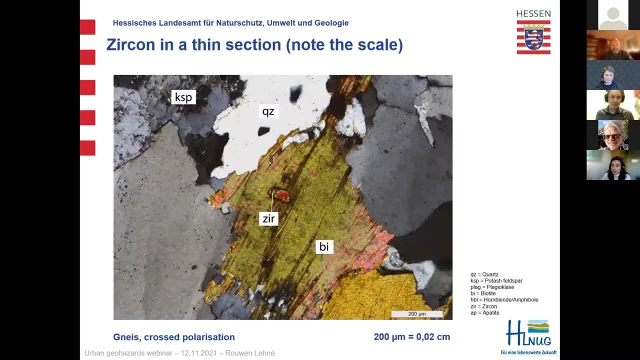 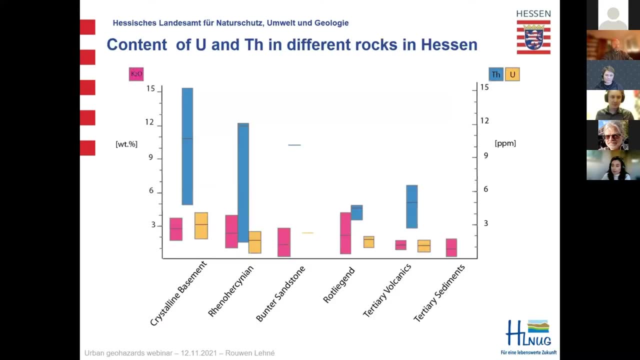 the same with another thin section where you can see the zircon there. and if we know about these minerals and if we know about their occurrence in the rocks, then we can do some statistics and see what is happening on the surface of the surface of the ge aby, the last on the recently mentioned 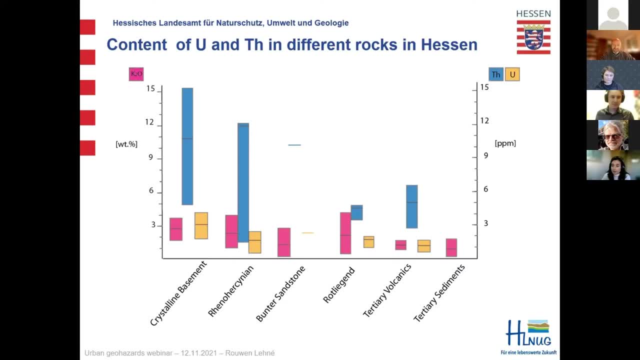 geochemical data. the geochemical data, the geochemical data is that we, the geochemical data, the geochemical database, is hosting a lot of uranium in the geochemical data is hosting a lot of uranium, a lot of thorium, like, uh, the rocks and the in the rainy shield. 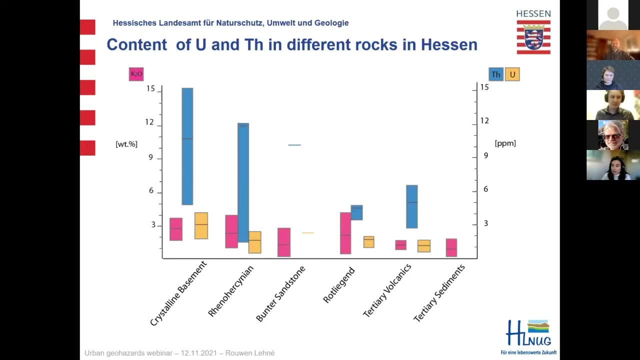 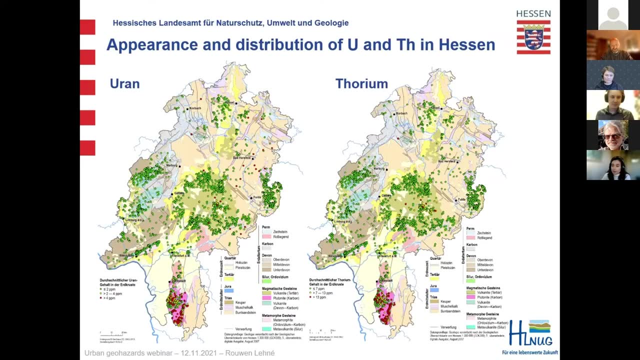 it's a bit less it's, it's quite. it's quite okay in the sandstone, but uh, and in the tertiary sediments, but the, the wood ligand and the tertiary organics, they also. I was talking about the geochemical database. this is how it looks like if you bring it on a map. 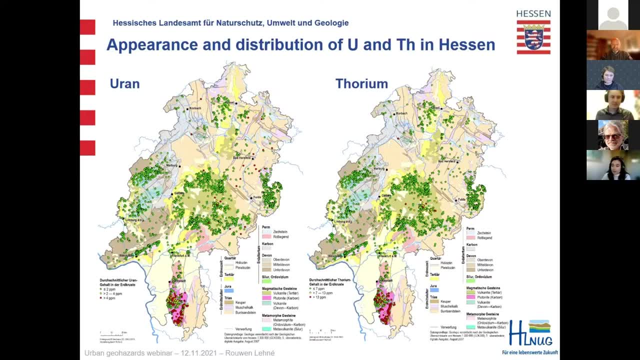 every point is representing a sample and every sample has been analyzed for uranium, thorium and others, and most of them- most of the samples- do not show any problems in terms of their concentration of uranium and thorium- the average concentration of uranium in the earth's crust. 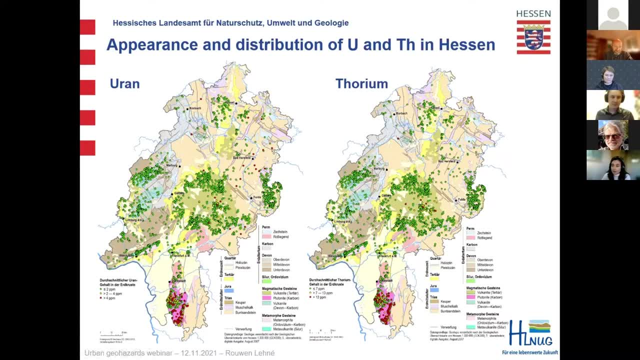 is two to four ppm and that's given in yellow. if the concentration is less it's green, and if it's above the average it's it's red. so you see on the left the uranium. yeah, it's. maybe this may be a topic in the southern part of the federal state in the 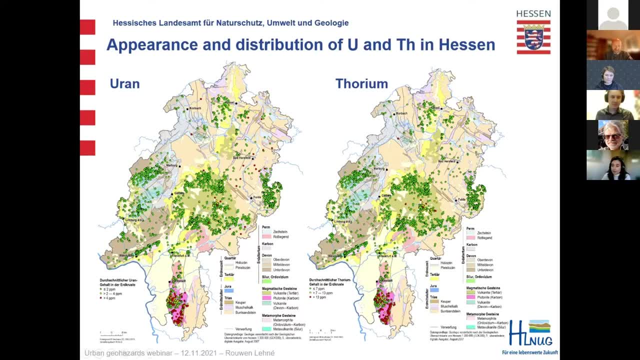 odenwald mountains, where we do have the crystalline rocks, and here and there and parts of eastern hesse also. some samples show higher concentrations of uranium. it's comparable with thorium, so the average in the earth's crust is 7 to 30 ppm, 13 ppm, sorry again. yellow, green is less and red is higher. 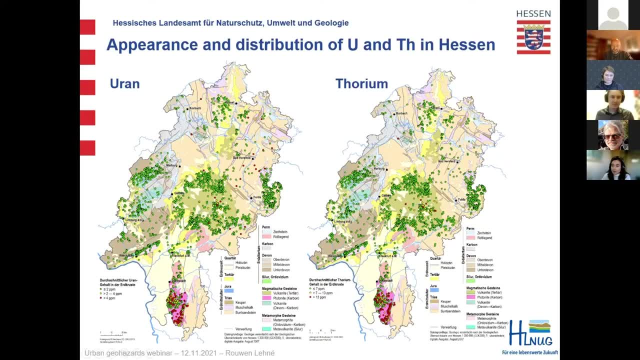 and still we are focusing on the odenwald mountains down there and parts of the Vogelsberg volcanic complex. yeah, but if we look at the odenwald mountains, we see that they are not as dense as the odenwald mountains. yeah, but if we look at the odenwald mountains, we see that they are not as dense as the odenwald mountains.